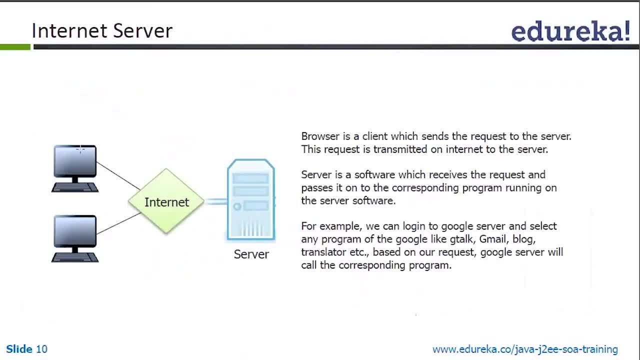 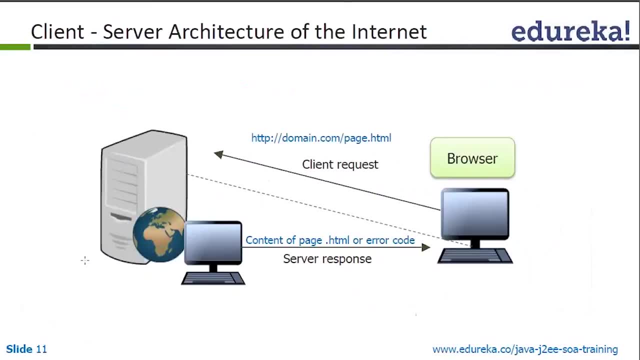 Now, if you look at, like you know, the internet server- basically you have a client or your browser, then you have internet. from there, it connects to the server and responds back. Okay, Now let's look at a web technology example. 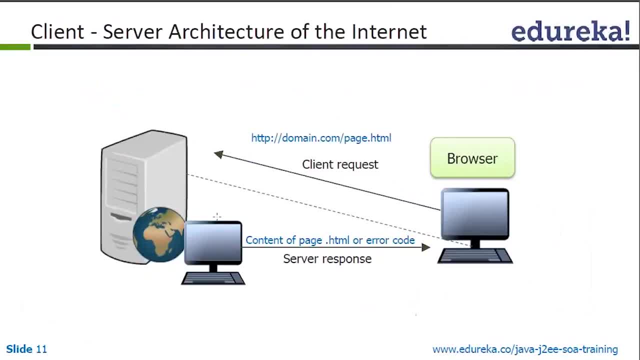 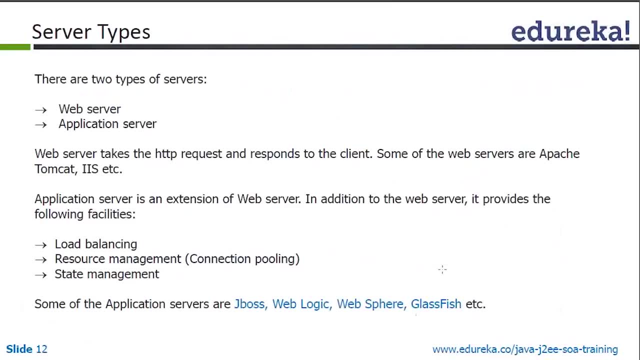 Let's look at a web technology example. Again, the same thing in a different way. right From the browser, the client gets requested to the server. it processes and responds back to the browser. Now let's look at the different kind of servers we have. right. 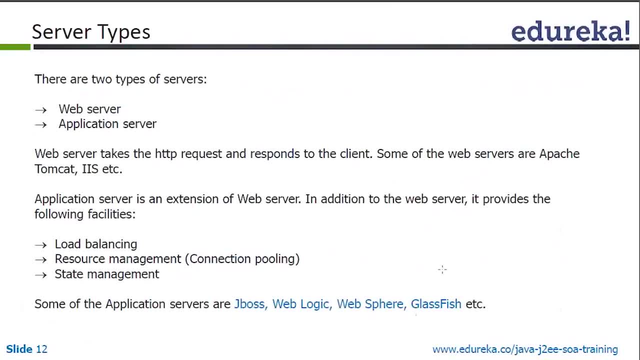 So there are two kinds of servers. One is a web server, another one is an application server. A web server. basically, what it does is it takes the request, routes the request to the particular program. It's like you know, you go to an office. there you will find a receptionist and he or she will, like you know, route to you means guide you to the correct person, right. 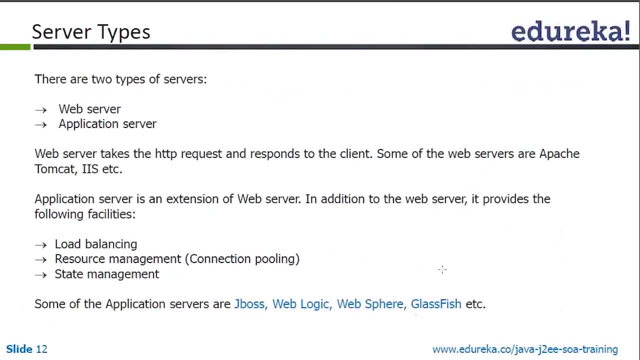 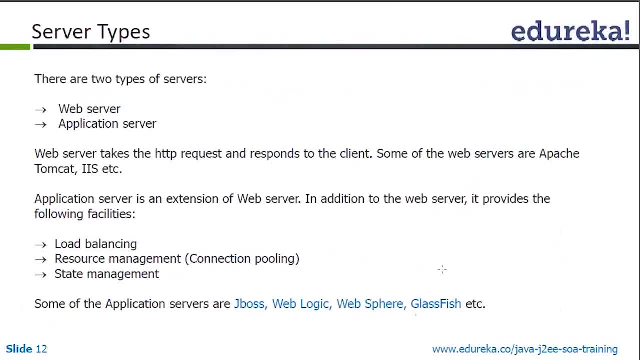 a huge amount of requests, like you know. some 10,000, a million requests are coming out for a web server, for a website. Then if you use only one system, it will be, like you know, it will be difficult to manage because the performance will go down. 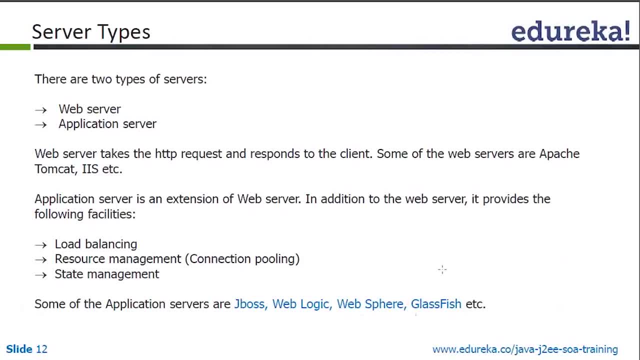 One million requests. at the same time, the performance of the system will definitely go down. In that case, what you have to do is you have to distribute- Okay, The application into so many things. okay, so many machines. that will balance it. 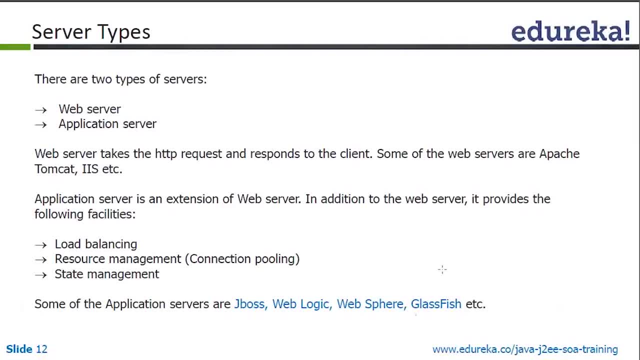 Like you know, maybe 10,: first 10 requests in one system, second, 10 requests in the second system, third 10 requests Like that. it uses round-robin technique to assign Then. so there is something called connection pooling. 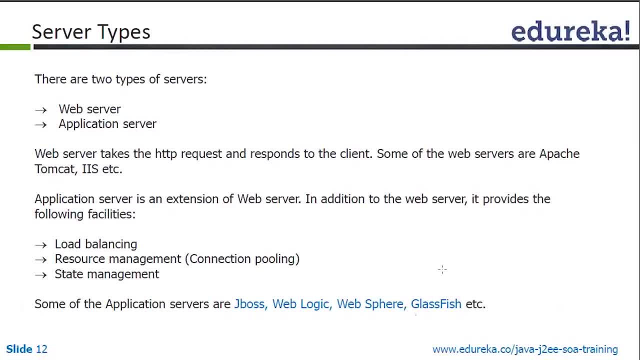 Okay. Connection pooling is basically: you have 10 resources. Somebody requests for it. One resource is gone. One resource is given. The resource pool will have nine resources. If somebody else asks for it, one more resource is given. Eight resources are left over in the resource pool. 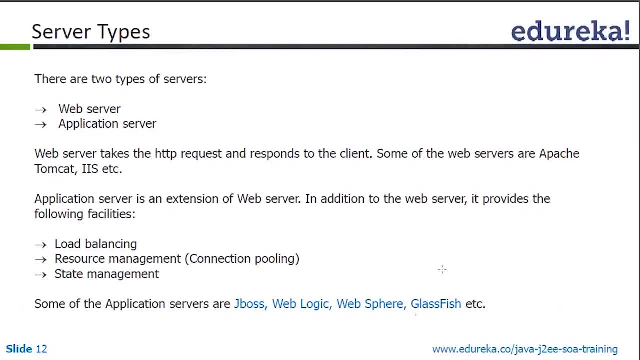 Then, like you know, somebody is done with the job, they will return it back to you. Like you know, eight, Then it will be nine. resources will be left over. Now you have one more resource, They will give it back. 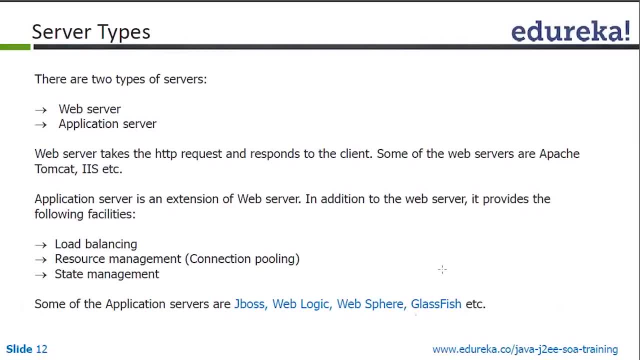 So, like you know, it will become 10 resources. It's basically back. It's like a bank kind of Resource pool is like a bank. So you deposit and withdraw, deposit and withdraw. That's all is a concept of connection pooling. 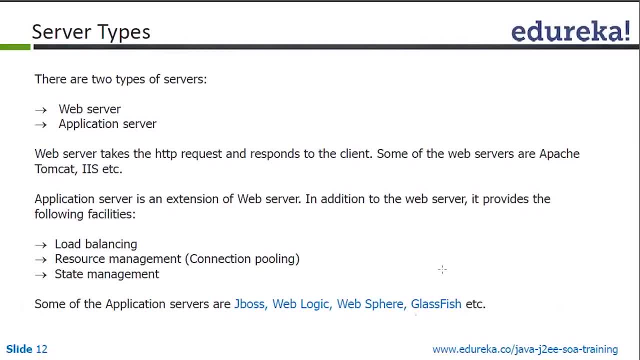 There is something called state management. State management is that? state management is it will store the state of the user Right, For example, if you are, like you know, using, Using the shopping cart. basically, there is something like you know, whatever the 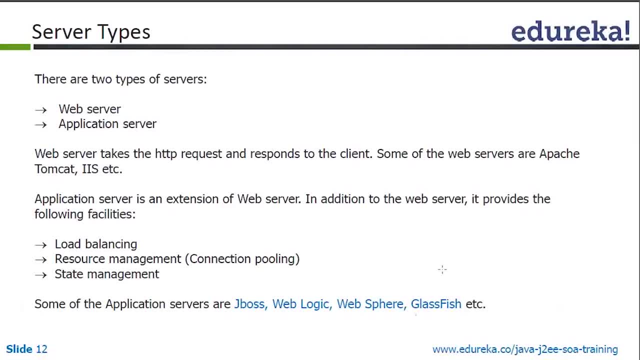 selection you make it it should store on the shopping cart, Right? So otherwise, like you know, it will be difficult Right Now. there are some more technologies that are provided by the application server, That is, EJB. Enterprise Java Beans is those technology, and another technology, JMS Java. 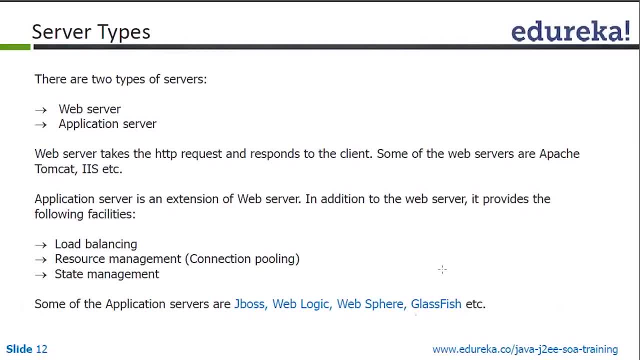 Messaging Server. This is not possible in web server. It is only possible in an application server. Okay, So these are the major differences between the web server and application server. Some of the examples of the web server is IIS, Internet Information Service and Apache. 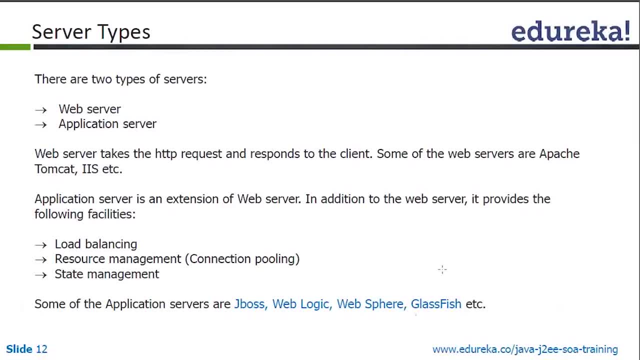 Tomcat, Right, Then in like application server. you have so many JBoss. is there Glassfish? is there, Right? WebLogic, WebSphere, WebLogic, WebSphere. So many things are there. So the major difference between the web server and application server is okay, Apache, Tomcat. 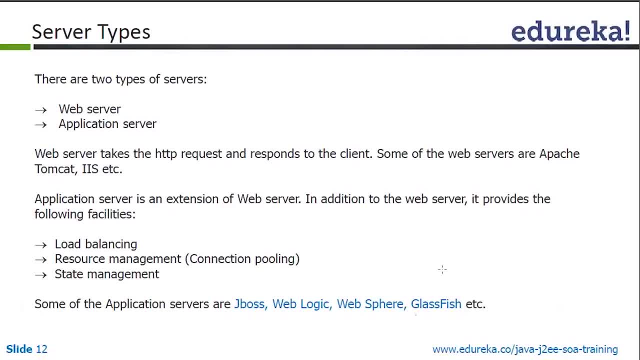 is a web server. Okay, So Apache Tomcat what it will do, like you know, it will keep on listening for the incoming request. Whenever there is a request, then it will route to the corresponding program Application server. a little beyond that, all the three facilities it provides. 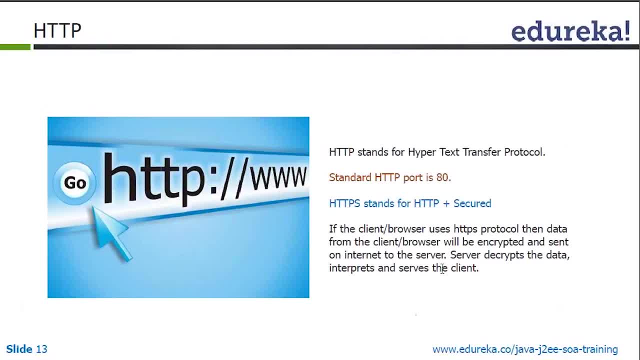 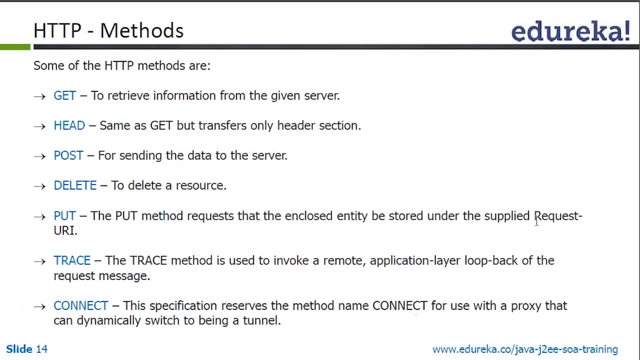 Okay, Okay Now, what is HTTP? HTTP is Transform, Hypertext Transfer Protocol, okay, and it is on port 80. It's a TCP IP protocol on port 80. is HTTP? Now a couple of methods of HTTP. you don't you'll not be using all, but you'll be using. 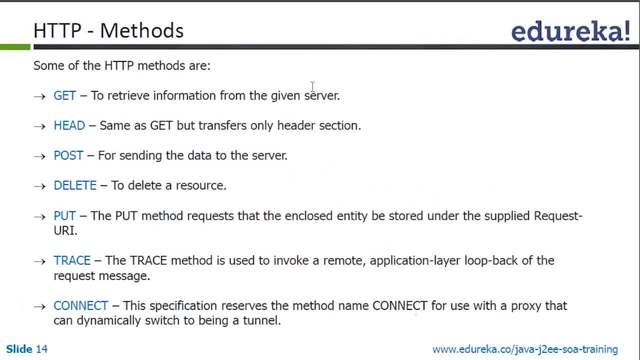 only two: GET and POST. Okay, You have GET, HEAD, POST, DELETE, PUT, RAISE, CONNECT so many. So, like you know, GET is, I'll tell you what is the difference between GET and POST. 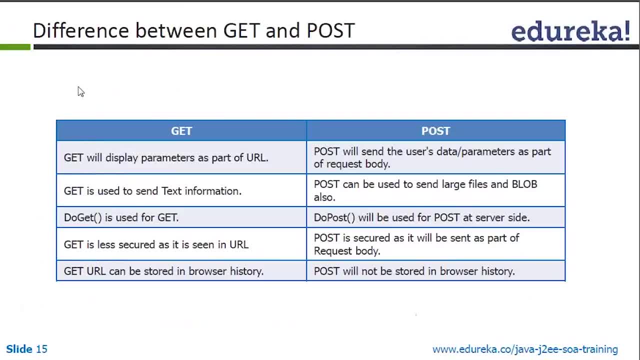 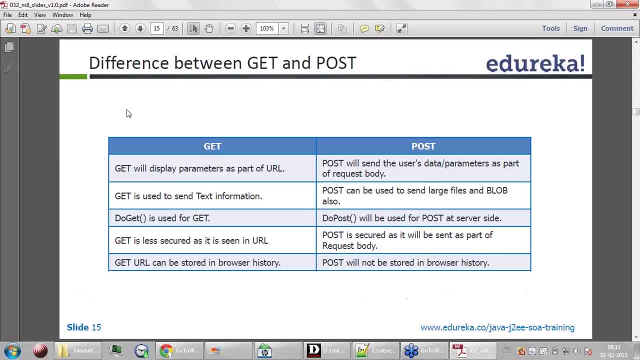 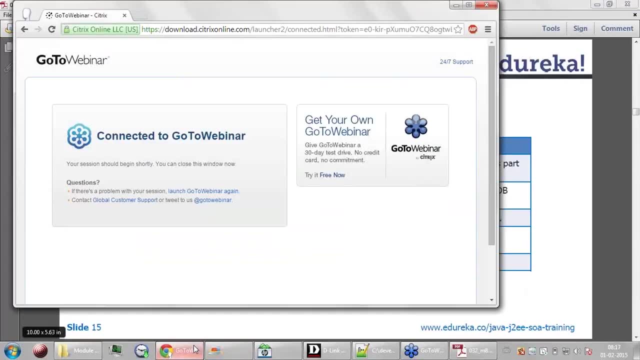 So just look at this slide, please, for 30 seconds. Now, the difference between GET and POST is that GET, okay, is a display part of URL. Now, if you look at like you know, I'll just give you. 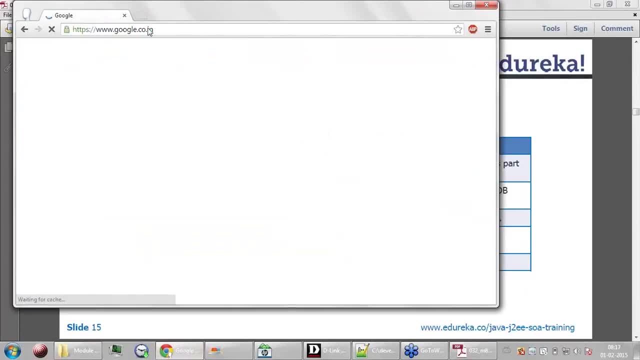 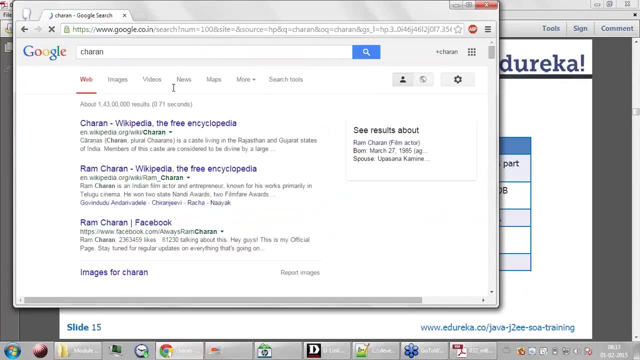 Okay, Okay, Okay, Okay Okay. If I type this, let's say that's a chart. So as part of, like you know, Googlecom, you will find as part of the URL, you'll find what is typed. 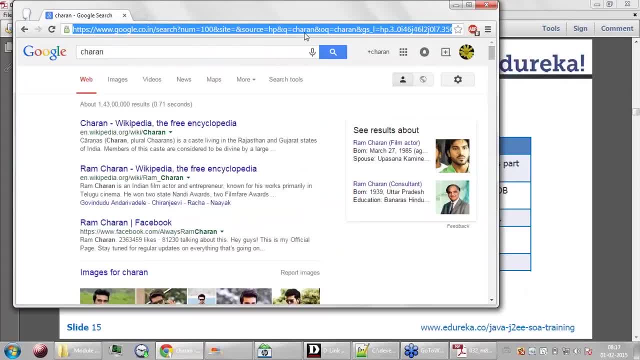 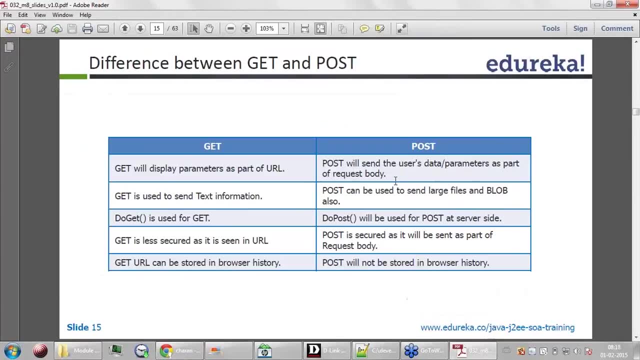 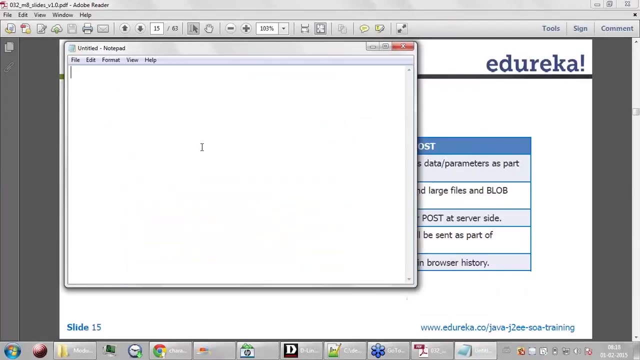 Okay, See, here you can see what is typed. That is a. it is going as a GET request POST will send the data or a parameter as part of the request body. See what happens is Okay, First the URL will go, then header will go, then data will go. 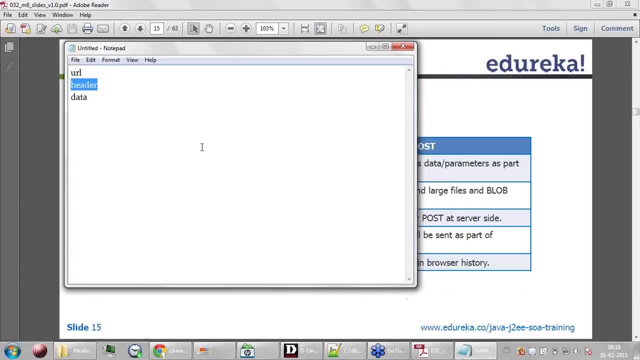 Okay, So header will have, like you know what is a browser where you have send which protocol it is using, all the header information about the browser and client. Okay, Okay, So the data of the machine and all those things will go as a part of the header. 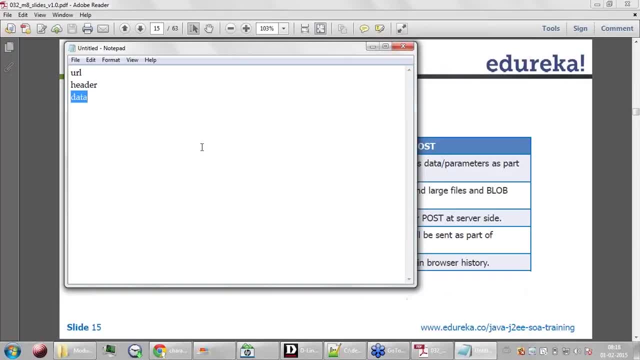 Data is, like you know, whatever you send the data from the POST method, So there are other ways, as the data can be sent as part of, like you know, as part of the URL itself. See here The data is going as part of the URL itself. 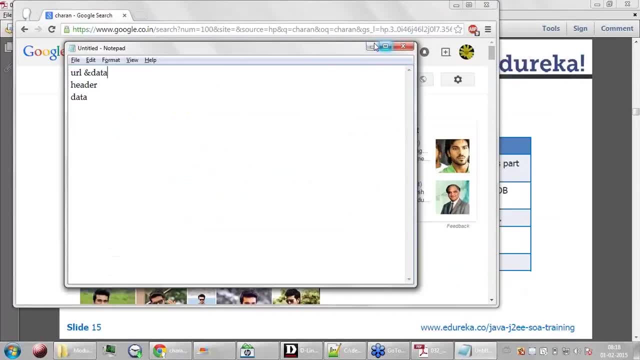 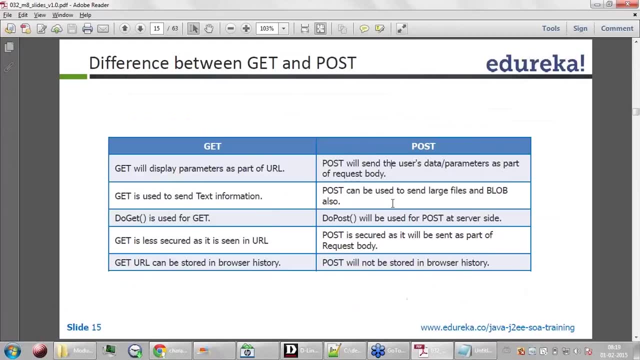 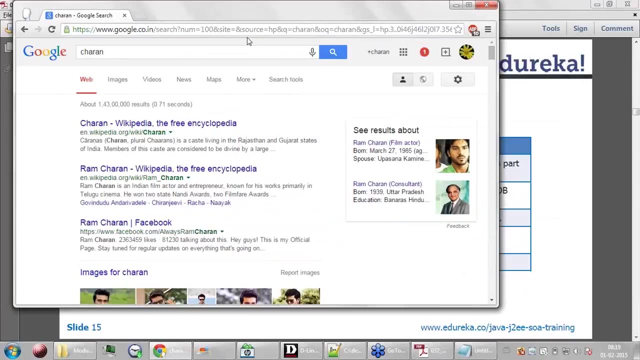 So that is the GET. If you don't, it doesn't go on as part of the URL, then it is POST, Okay, GET is used to send the text information. POST is, yeah, text only, So you cannot send the binary information over here. 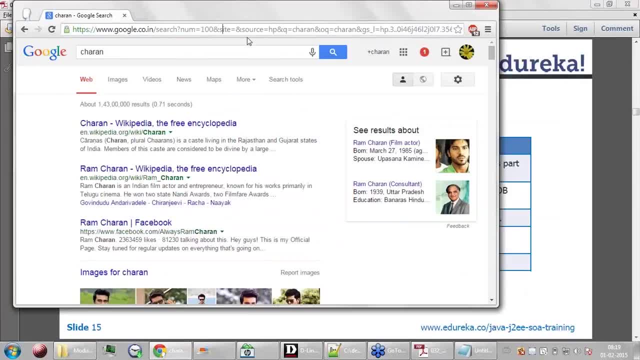 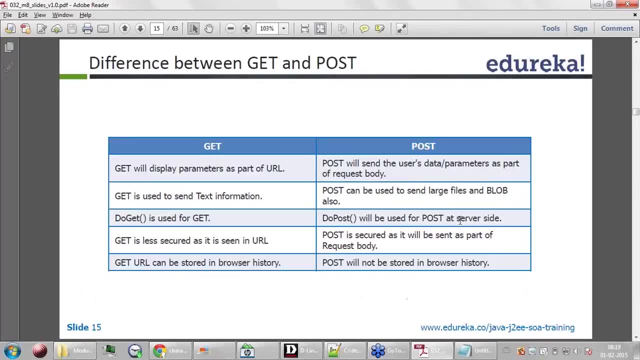 That is for GET, The POST. you can send the binary information, that is, binary large objects, Okay, So there is something called do GET, do POST available in servlet. We will look at those things. Okay, Then you have do GET is definitely less secure. 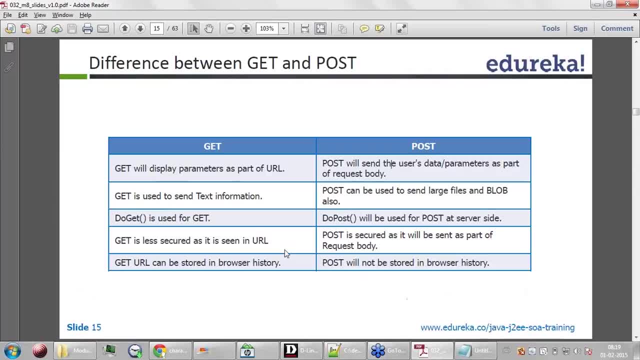 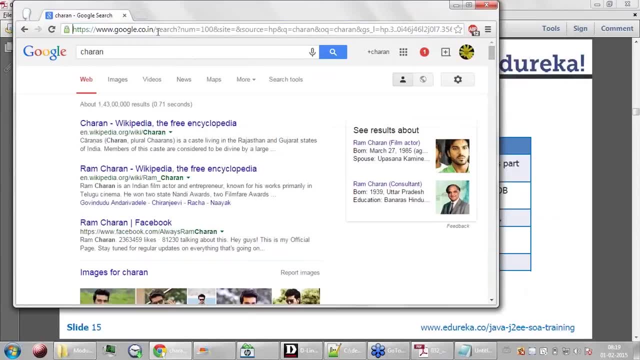 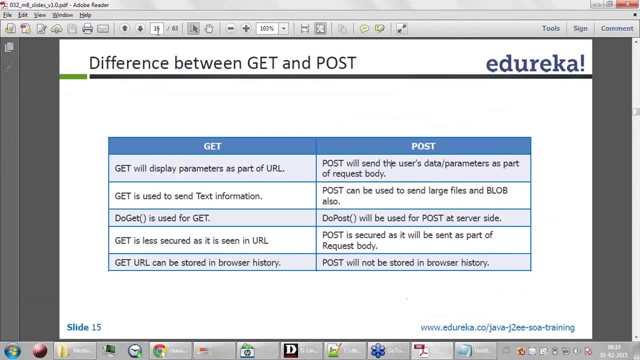 Why? Because see, whatever the data you are sending to the server, it is clearly seen Right, Hacking becomes easy. It is definitely less secure Right, Whereas the PUT is, like you know, it is more secure. 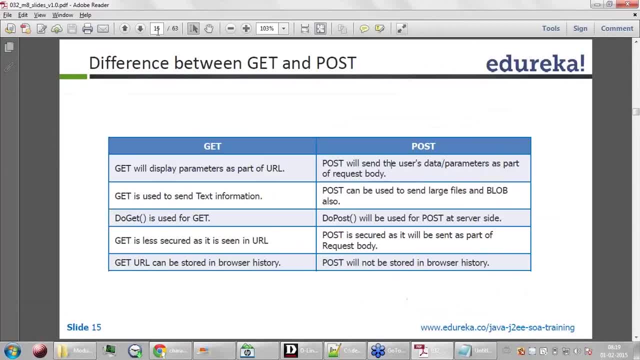 Basically, you are logging in one application- Okay, A web like banking application. You are providing your user ID and password, Correct. So in that case, what you do, You go as user ID and password. So it will definitely go as a POST method because it is easy. 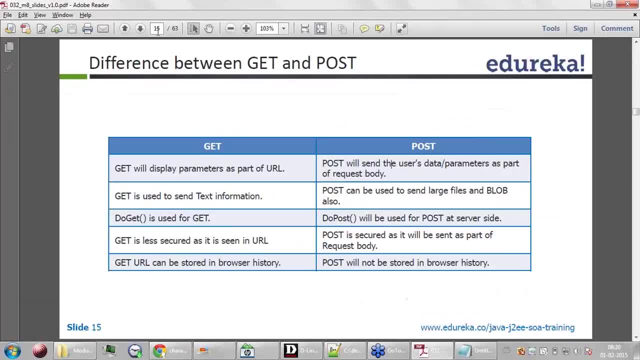 Right, It is like you know. it is more secure. It is not. your user ID and password will not be seen as part of the URL. Right? Definitely, POST is much secure, Okay, So okay. Next is GET. URL can be stored in the browser. 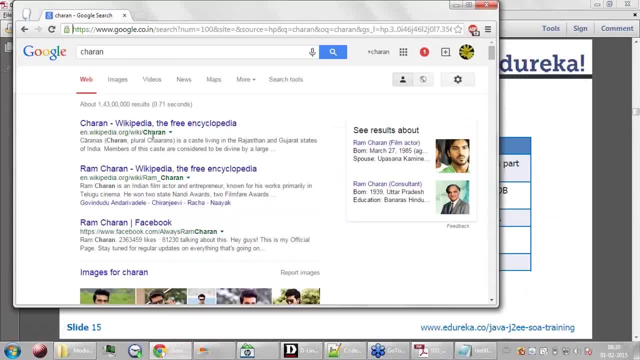 It can be stored in the browser history. So the thing is, if you look at this, like you know, whatever this, if you go to history, like you know browser history, So if you go to history, you will be able to see this website. 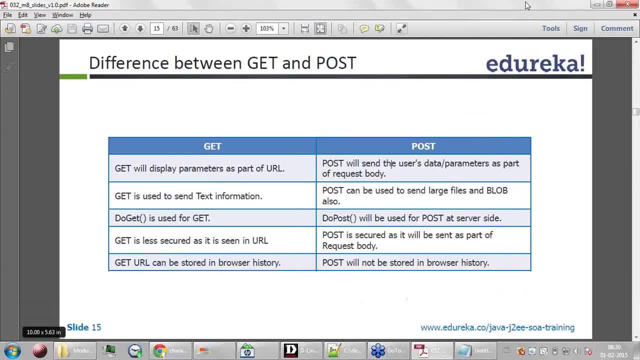 Okay, So the GET will be part of the history. POST will not be part of the browser history. That means what data it is going. it will not be seen as part of the browser history, Right? So that is what the GET and POST differences.